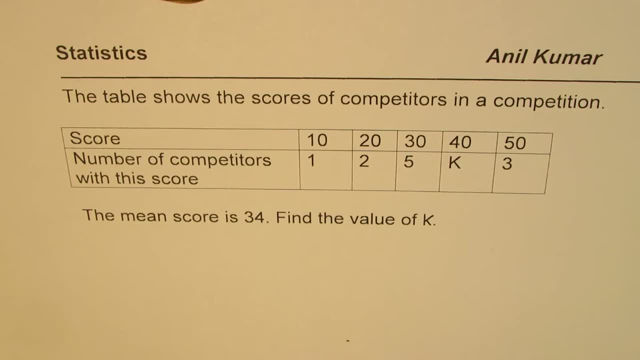 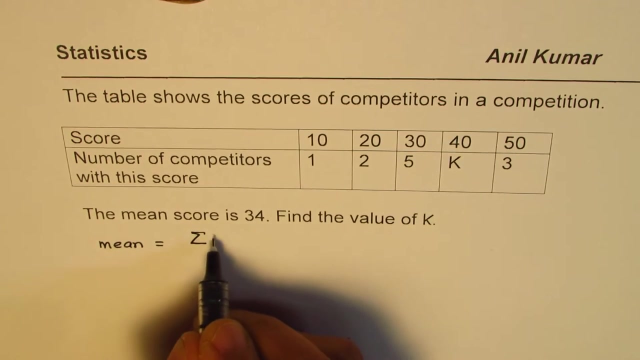 look into my suggestions Now in this particular case, since the mean score is given to us, which is 34, and we know mean is equal to the sum of frequency, with the number of items f of x divided by the sum of frequencies. That is how the mean is related. 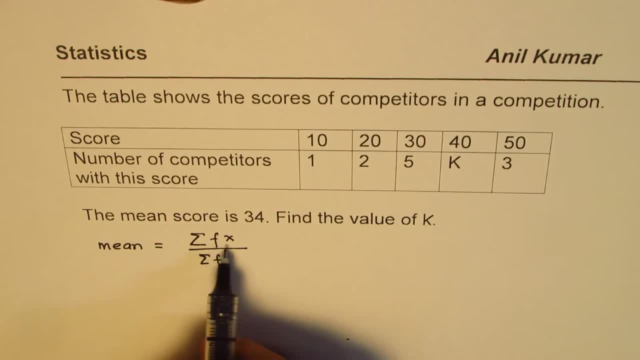 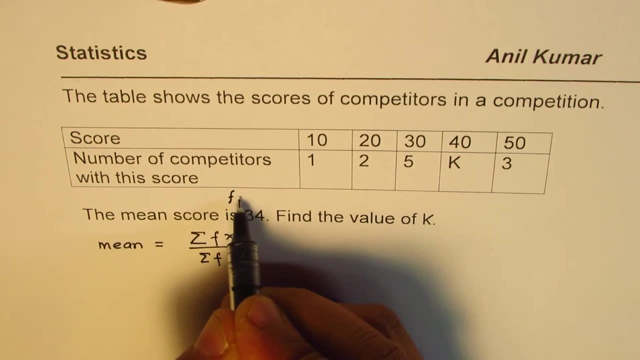 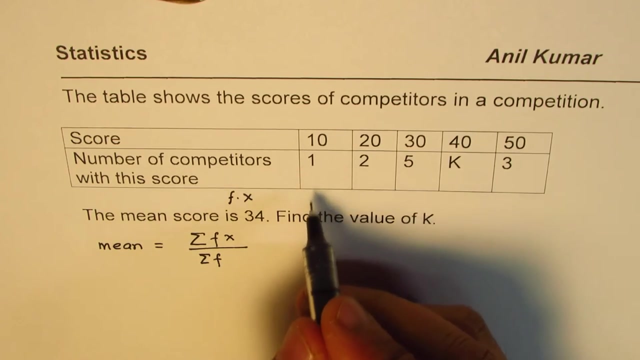 Now in this equation we can find the product, So we can add a column here which is f of x. Let's add this column and then we'll find the sum and use this formula. So 10 times 1 is 10,. 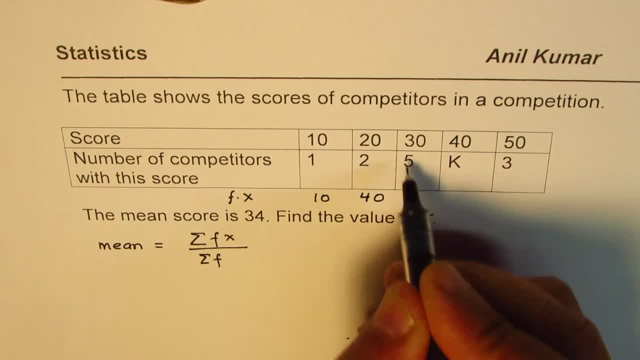 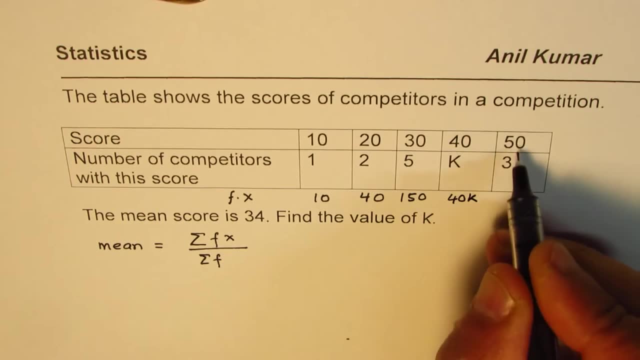 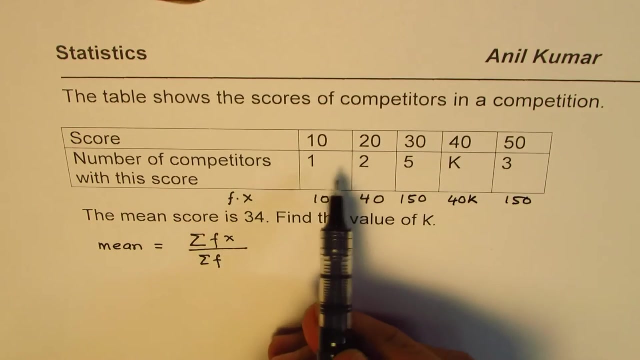 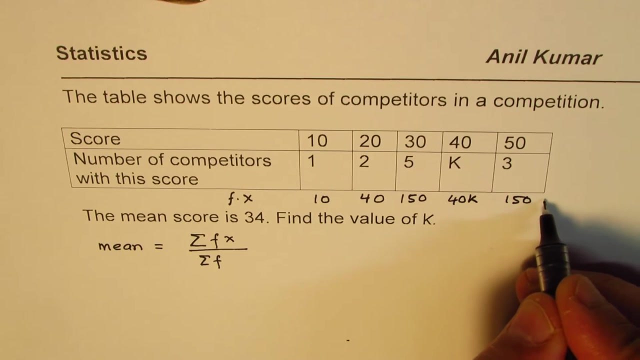 2 times 20 is 40,. 5 times 30 is 150. Here we get 40 K and here we have 150,. right, So that is the column which shows product of frequency with the score In this particular case. right, so that becomes the product, and some of these values is equal to. 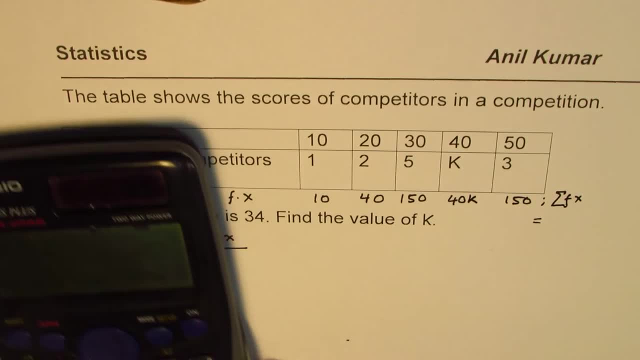 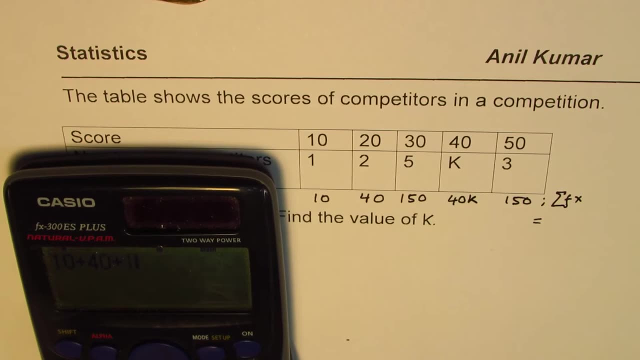 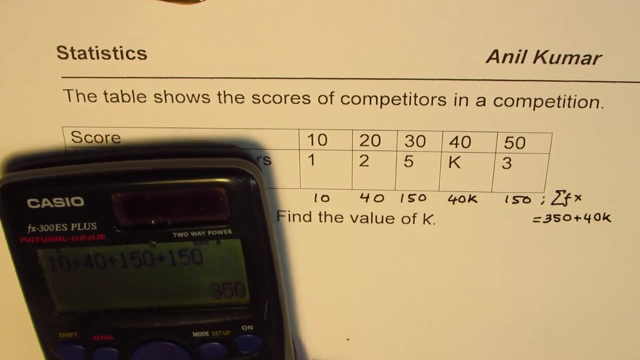 let's find the sum here, So, which is 10 plus 40 plus 150 plus 150, which is equal to 350.. So we plus 40 k, is that okay? so that is the sum which we get of frequency times, the scores, right. 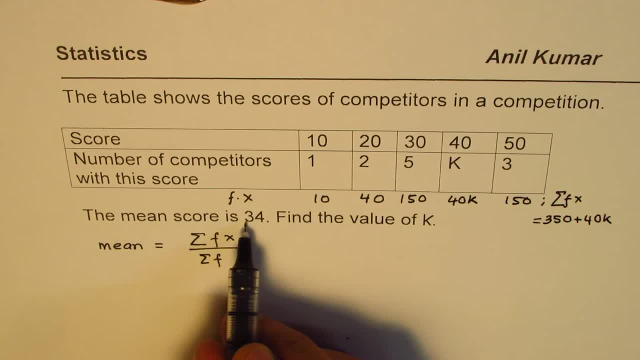 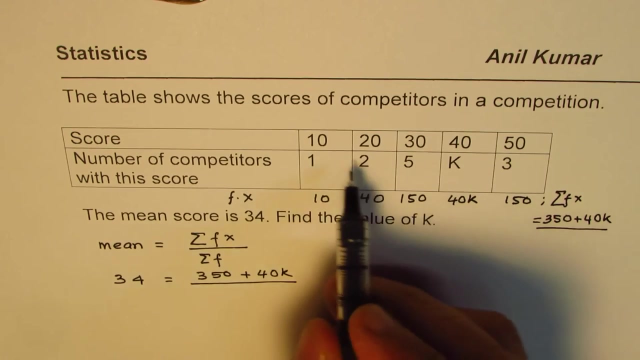 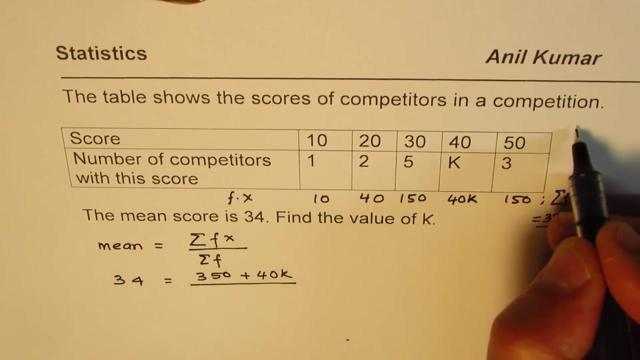 so in this formula we can write: mean, which is given to us as 34, equals to that sum which we just calculated, which is 350 plus 40 k divided by the sum of frequencies. so sum of frequencies, we can combine this. let's find the total here for frequency, so it is 1 plus 2 plus 5 plus 3, which is 3 and 3, 6, 6 and 5, 11, which is 11.